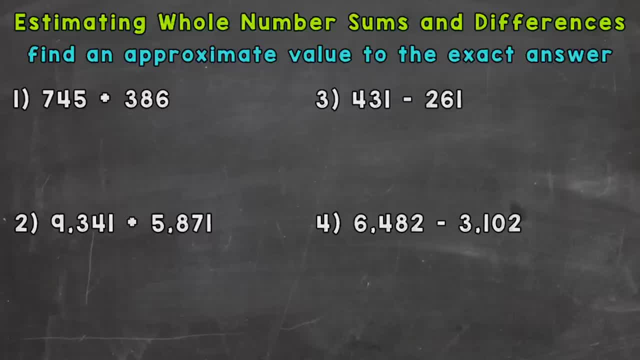 means we're going to round to the greatest valued place. So the place furthest to the left. In the case of number one, it's going to be the hundreds place here and the hundreds place here. So 745, is it closer to 700 or 800?? Well, it rounds to 700. And then 386 rounds to 400. So we would 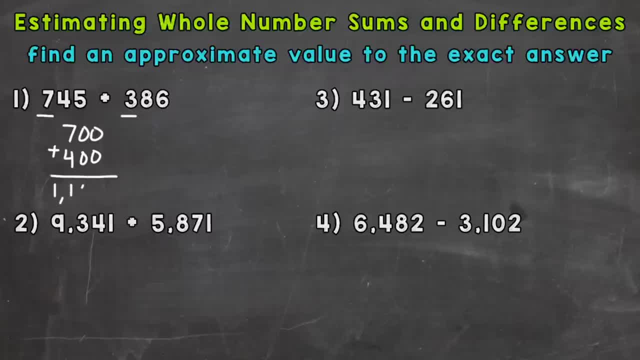 add these for our estimate and get 1100.. So we could say that 745 is approximately 1100.. So this little squiggly equal sign there means approximately. Now the actual exact answer to number one is 1131.. So you could see that our estimate was pretty close to that estimate. 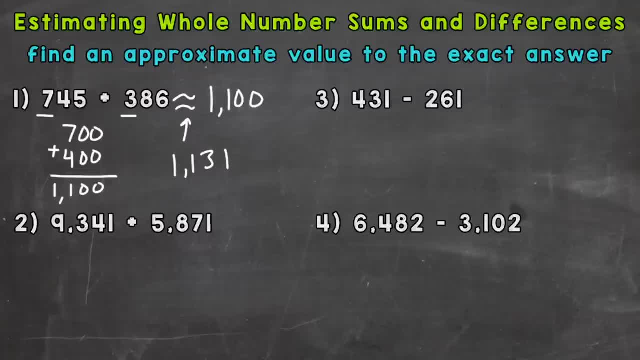 On to number two, where we have 9341 plus 5871.. So let's use front end estimation again here. So thousands place, So 9341 rounds to 9000. And 5871 rounds to 6000. And we get an estimate of 15,000 there. Now the actual. so let me put our estimate here. 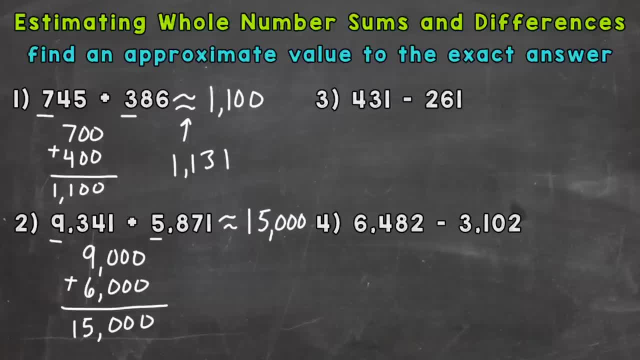 and then I'll do the actual answer. So the actual exact answer is 15,212.. So again, pretty close to that exact answer. On to number three here, where we have 431 minus 261.. Now I'm going to go through a couple of strategies. for this one I'll do front end estimation. 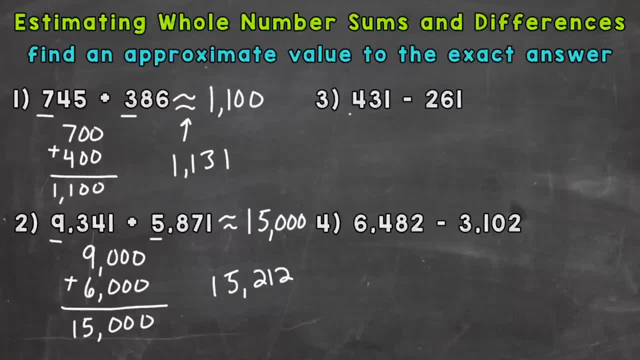 and then another strategy. So, front end, we'll go to the hundreds place. So 431 is going to round to 400.. And we are going to subtract, well, 261 rounds to 300.. So our estimate is going to be 100. 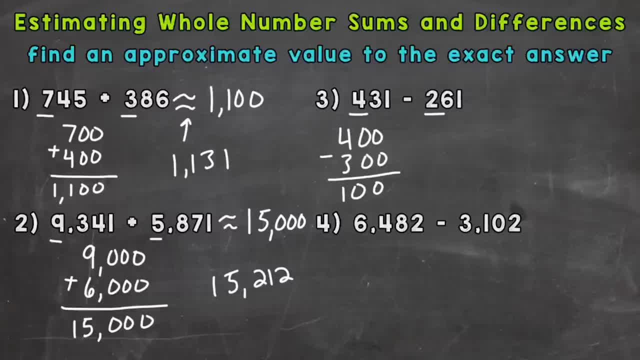 for front end estimation. I will show you another strategy here that's going to get us a close to that exact answer. So we're going to go through a couple of strategies for this one Closer estimate. Now I do want to say, when it comes to estimating, there are no set rules that 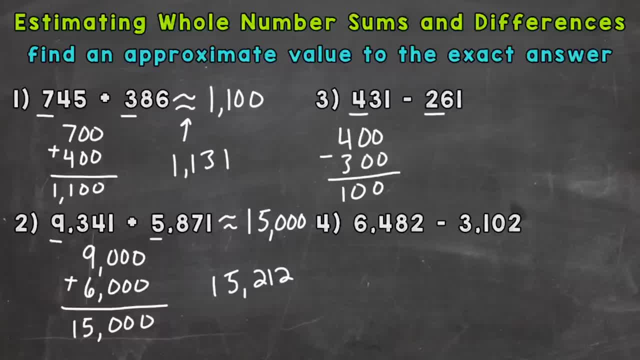 you have to follow. There are a bunch of different strategies, So whatever works best for you. The closer you round your numbers to the original problem, the better your estimate is going to be. So let's try a different strategy here, where we're going to take a look at rounding these. 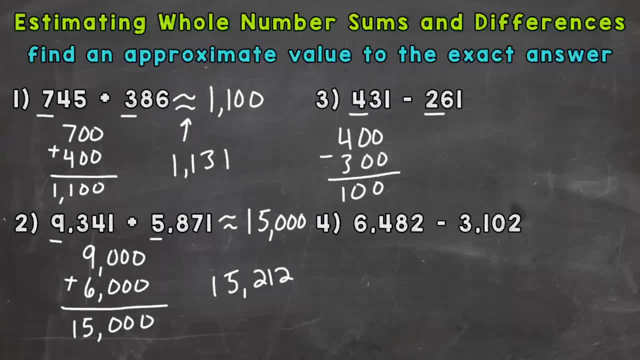 to closer numbers. So, for example, 431, we rounded to the hundreds place and we rounded to 400.. Well, another strategy we could use: we could take a look at the halfway or midpoint there. So instead of asking ourselves: is 431? 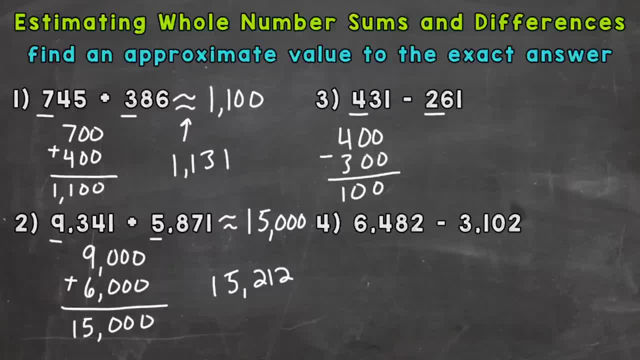 closer to 400 or 500,. we could take a look at 450,, because 431 is closer to 450 than it is to either one of those hundreds place, 400 or 500. So let's round to 450. And we'll do the same thing. 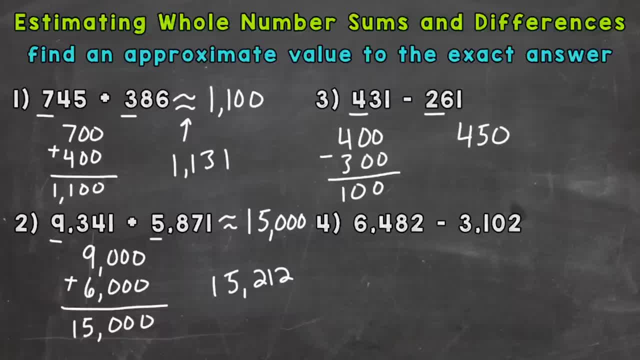 for 260.. that's actually closer to 250. then it is 200 or 300 if we were to round to the hundreds place. so let's use 250 for that one subtract and we get an estimate of 200. so notice how our two estimates differ. now neither one is incorrect, but 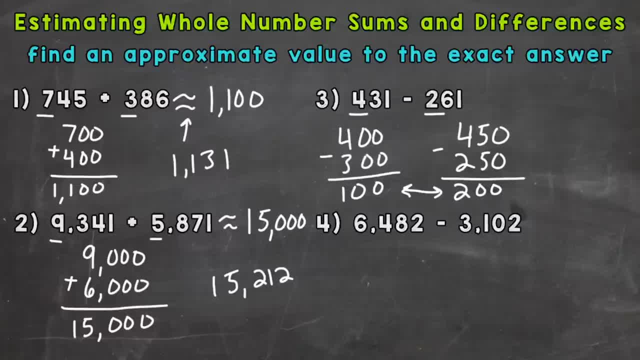 one is going to be closer than the other. so the actual, exact answer, I'll put an actual equal sign: there is going to be 170, so 200 is closer to 170, then 100 is. so our second estimate: there was a better, closer estimate and that is: 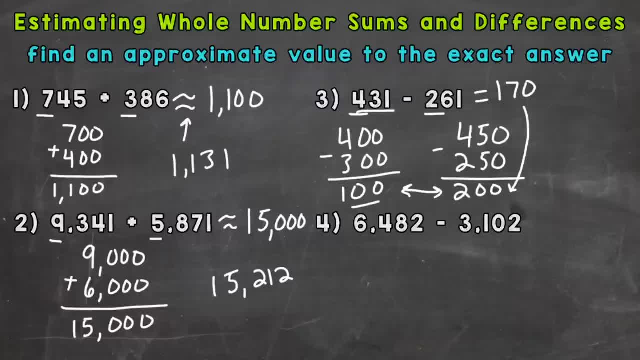 because 450 is closer to 431. these are closer than 400 would be right there. and we got our second estimate: this is closer to 50 be and 261 is closer to 250 than it is to 300. so we rounded closer to the. 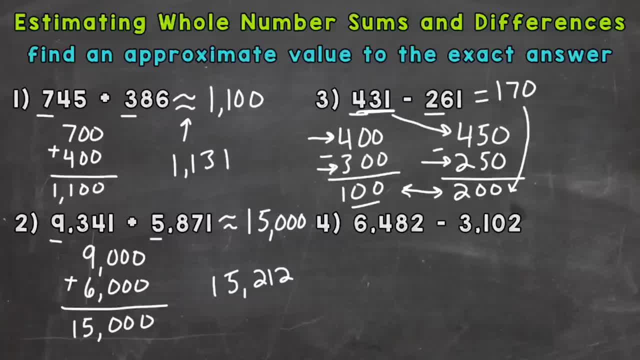 original problem for our second estimate. and again, rounding closer to the original problem gives a closer estimate. so let's try number four, and we'll use two strategies here. we'll use the front end estimation and then the half or midpoint. so let's take a look at the thousands place here: six thousand four.